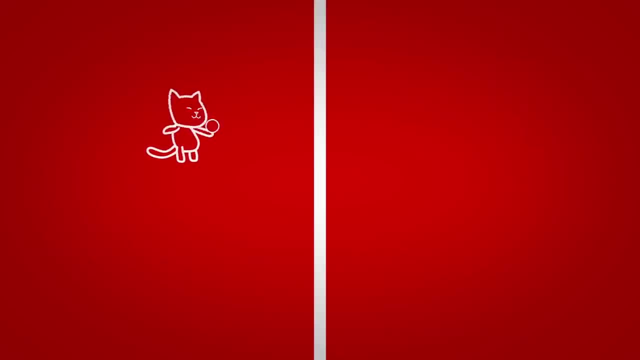 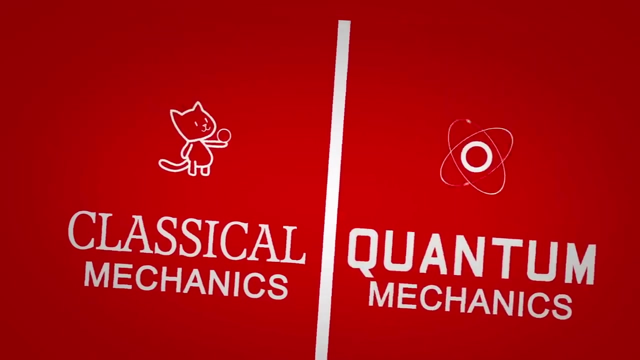 you see around you all the time. The everyday world you know and love behaves according to the laws of classical mechanics, But systems on the scale of atoms behave according to the laws of quantum mechanics. This quantum world turns out to be a very strange place. 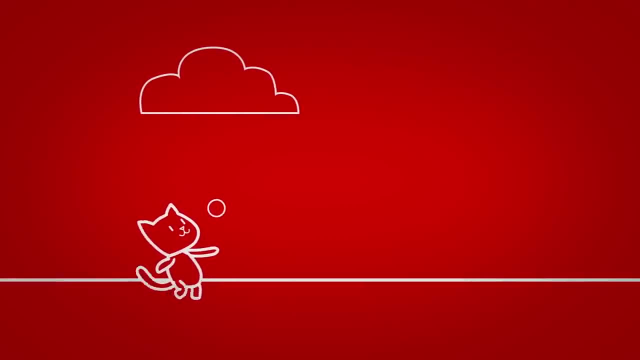 An illustration of quantum strangeness is given by a famous thought experiment: Schrodinger's cat. A physicist who doesn't particularly like cats puts a cat in a box along with a bomb that has a 50% chance of blowing up after the lid is closed. 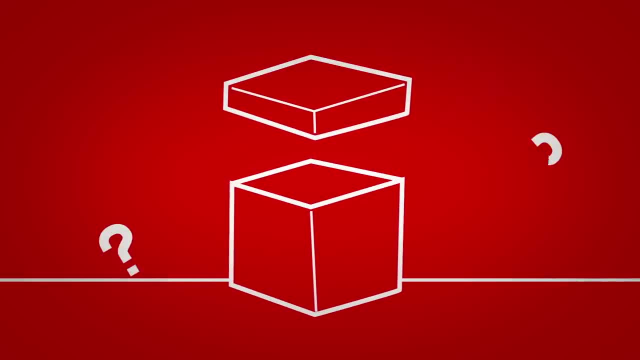 Until we reopen the lid, there is no way of knowing whether the bomb exploded or not, and thus no way of knowing if the cat is alive or dead. In quantum physics, we could say that before our observation the cat was in a superposition state. 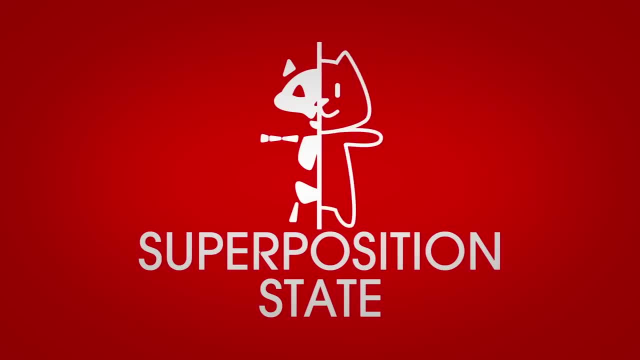 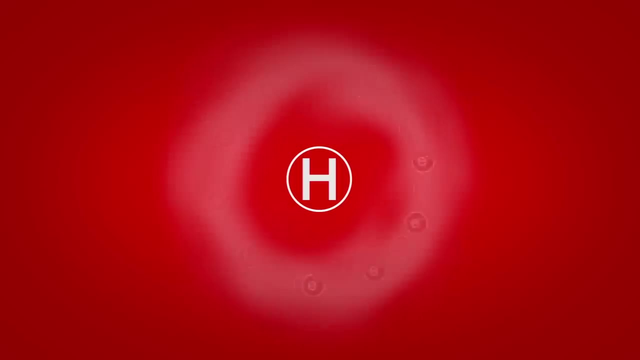 It was neither alive nor dead, but rather in a mixture of both possibilities, with a 50% chance for each. The same sort of thing happens to physical systems at quantum scales, like an electron orbiting in a hydrogen atom. The electron isn't really orbiting at all. It's sort of everywhere in space all at once, with more of a probability of being at some places than others, And it's only after we measure its position that we can pinpoint where it is at that moment. A lot like how we didn't know whether the cat was alive or dead. 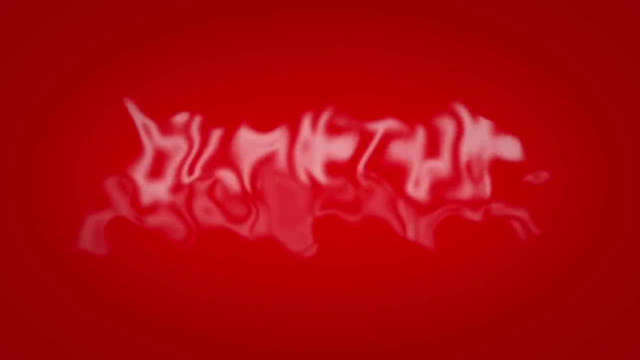 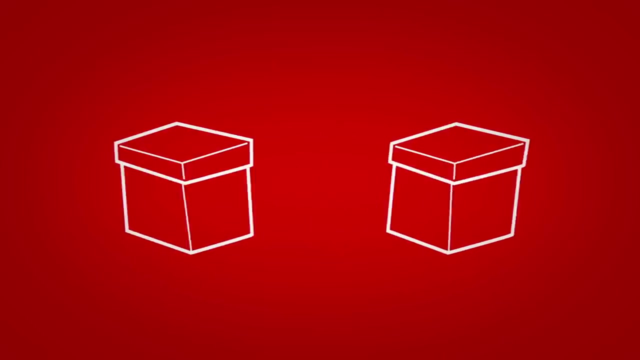 until we opened the box. This brings us to the strange and beautiful phenomenon of quantum entanglement. Suppose that instead of one cat in a box, we have two cats in two different boxes. If we repeat the Schrödinger's cat experiment with this pair of cats, 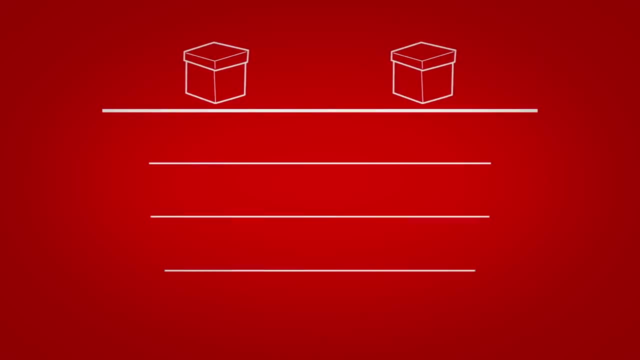 the outcome of the experiment can be one of four possibilities. Either both cats will be alive, or both will be dead, or one will be alive and the other dead, or vice versa. The system of both cats is again in a superposition state. 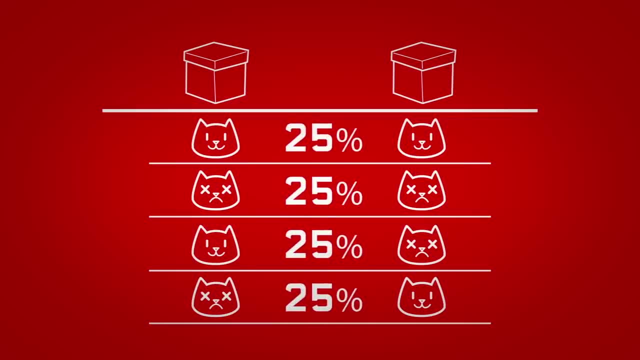 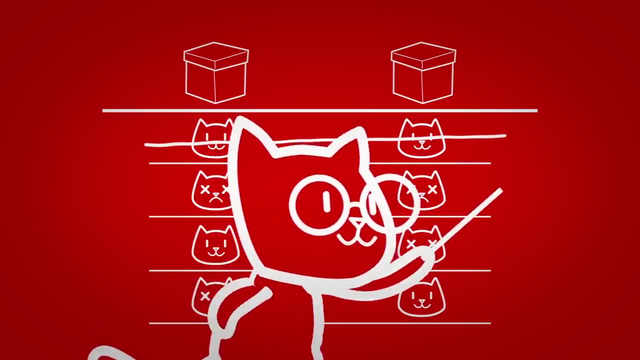 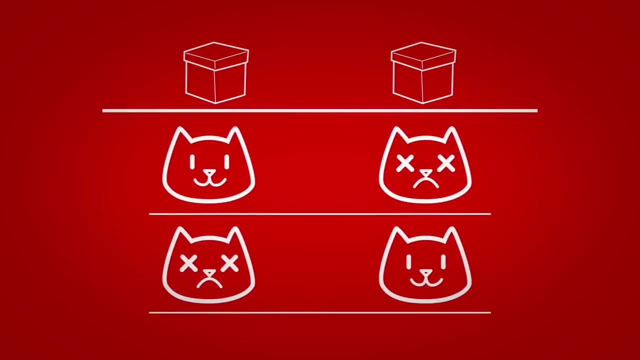 with each outcome having a 25% chance rather than 50%. But here's the cool thing: Quantum mechanics tells us it's possible to erase the both-cats-alive and both-cats-dead outcomes from the superposition state. In other words, there can be a two-cat system. 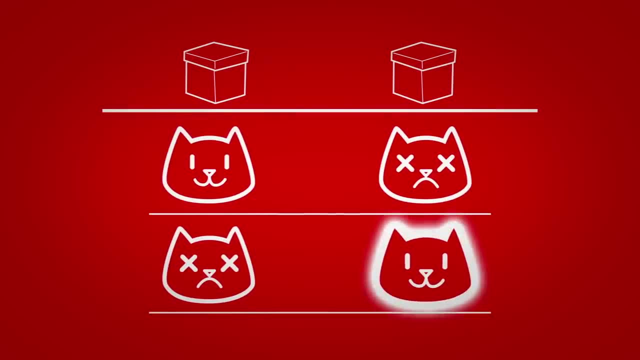 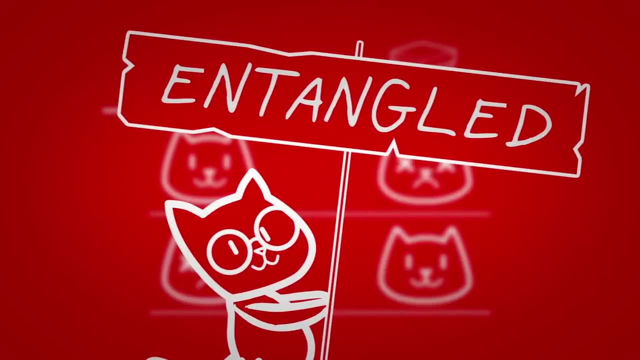 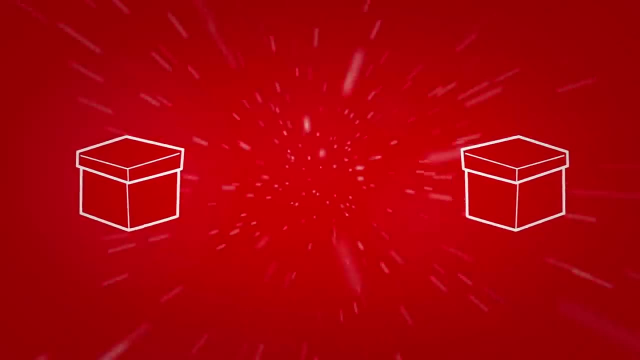 such that the outcome will always be one cat alive and the other cat dead. The technical term for this is that the states of the cats are entangled, But there's something truly mind-blowing about quantum entanglement. If you prepare the system of two cats in boxes in this entangled state.